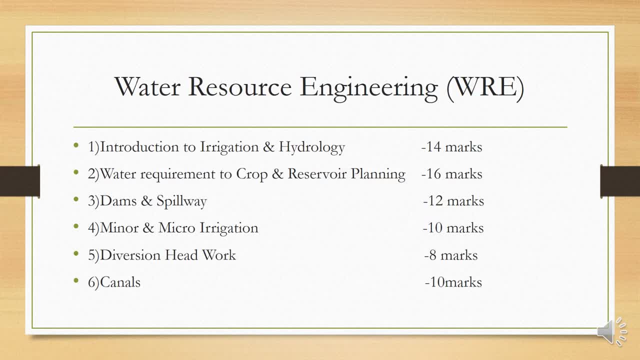 Okay, water resource engineering, having total 6 topic. First topic is on introduction to irrigation and hydrology. In this topic we will talk about irrigation and hydrology. In this first chapter we will learn about the definition of irrigation, then classification of irrigation, then what is hydrology, what is hydrological cycle, then what is rain gauge, what is runoff like, etc. 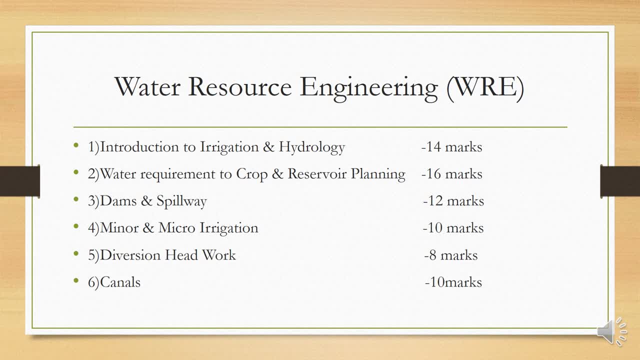 Okay, and first chapter is for potting marks. Your second chapter is water requirement to crop and reservoir planning. In this chapter we will learn about the different, different stops. requirement of water is different. Then again, delta duty, base period and some numerical depend on the delta base period and duty. 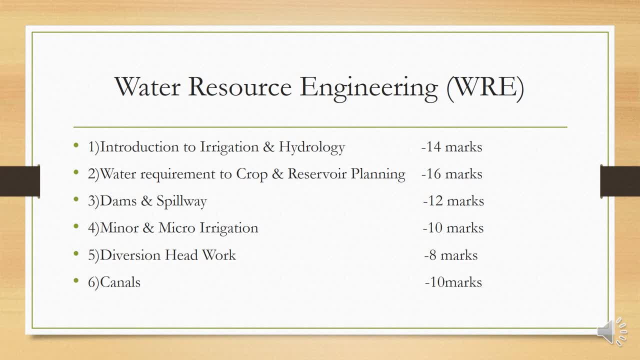 Then what is reservoir, planning or present? All this topic we will cover in a second chapter, and second chapter is for 16 marks. Your third chapter is dam and spillway. In this chapter we are having types of dams, The advantages about some dams, then spillway, types of spillway. 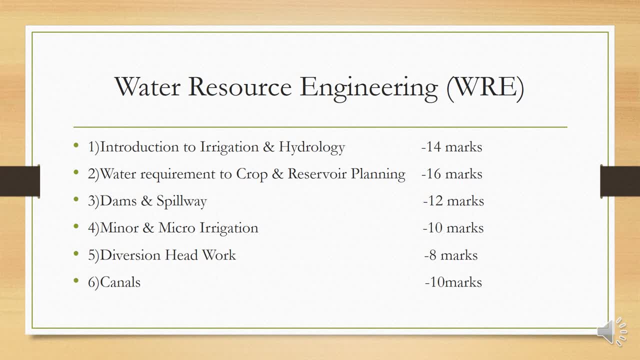 And third chapter is for 12 marks. Then fourth chapter is minor and micro education. This is for 10 marks, Then diversion headworks 8 marks, canal 10 marks. So total in this subject you are having 6 chapters. 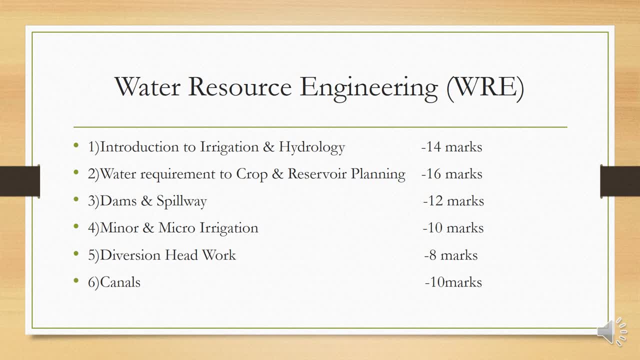 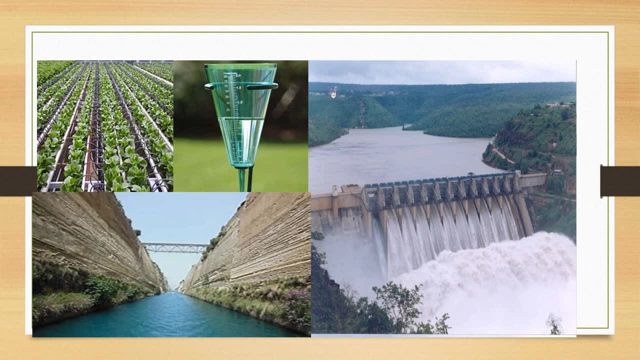 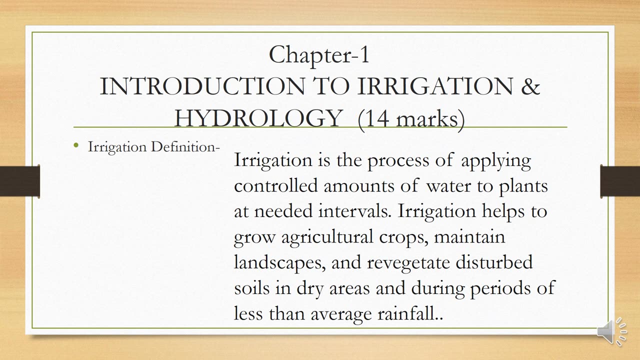 Okay, Let us start with our first chapter, that is, introduction to irrigation and hydrology. So first we will discuss about the definition of irrigation. What is irrigation? Irrigation is the process of applying control amount of water to the plant at needed intervals. 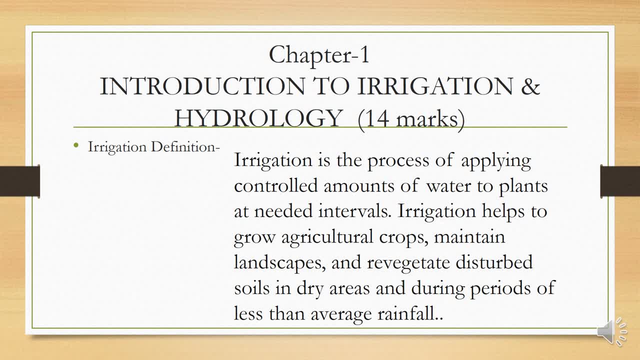 Irrigation helps to grow agriculture crop, maintain landscape and irrigate distributed soil in dry areas and during the period of less and average rainfall. In simple language, irrigation means applying of water to an agriculture area or a farm. Means all the farms and agriculture area for control amount of water to be applied. 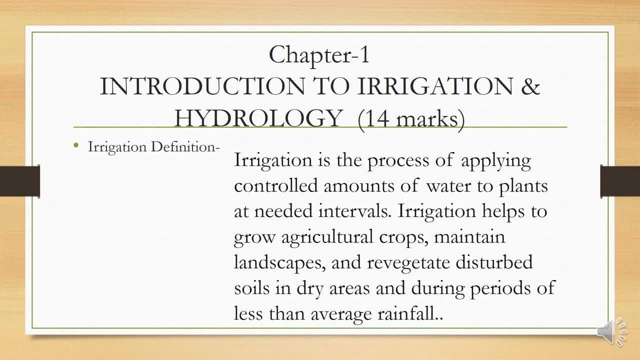 Water application means irrigation by using different methods of irrigation. Okay, Why this water is provided So that the crops of this plant can grow properly, And in the areas where rainfall is very less, we can provide water by using different types of irrigation. 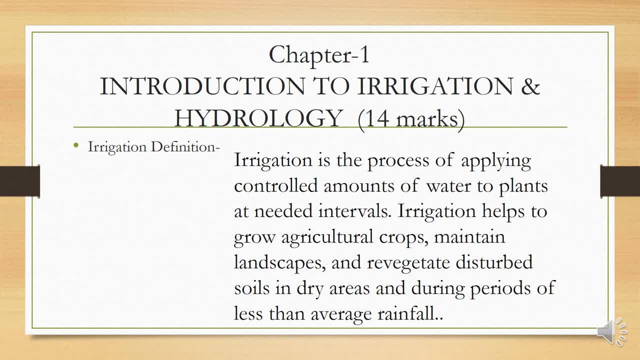 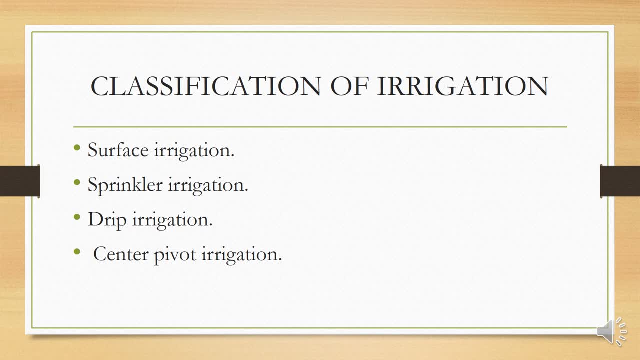 Okay, Now classification of irrigation. Irrigation is classified in 4 types. First one is surface irrigation, Then sprinkler irrigation, Then drip irrigation And last one is center fiber irrigation. Now, one by one, we will discuss about the each and every types of irrigation. 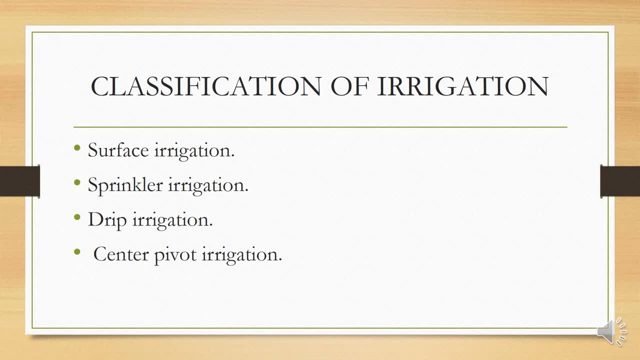 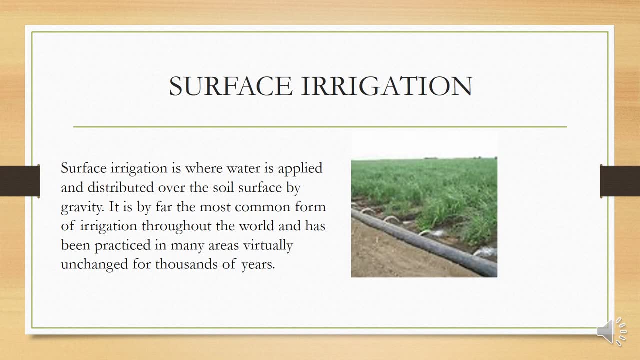 Okay, First is surface irrigation. Now, what is surface irrigation? Surface irrigation is where water is applied and distributed over the soil surface by the gravity. It is far the most common form of irrigation throughout the world And has been practiced in many areas virtually unchanged, for thousands of years. 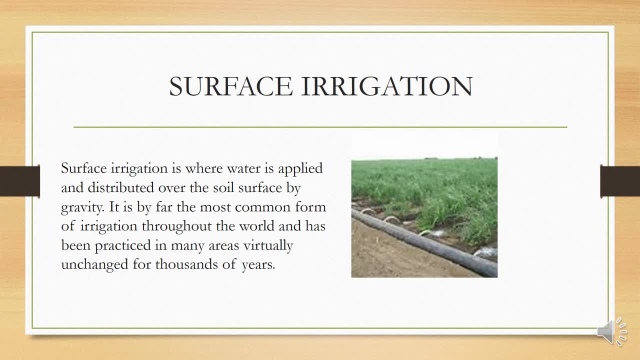 So this surface irrigation is a very basic type of irrigation. You must have seen it in the agriculture area or in the farms. So what is done in this? The farms create channels in horizontal form And water is provided by the force of gravity. 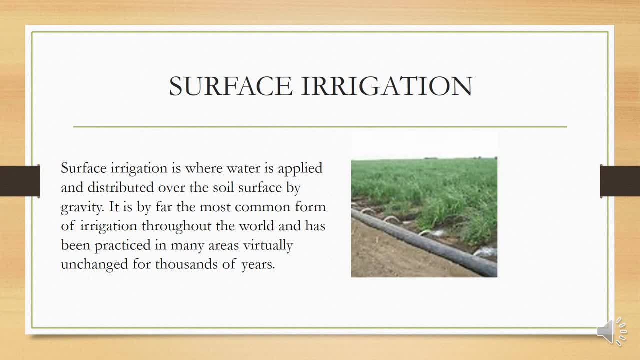 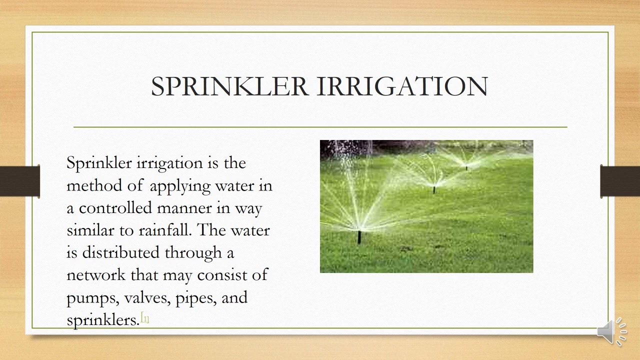 And, because of the slope, the water passes to the end. So this is a very basic type. This is a very common type of irrigation And it has been practiced for many years. Okay, Next is sprinkler irrigation. Sprinkler irrigation is the method of applying water in a controlled manner, in a way similar to rainfall. 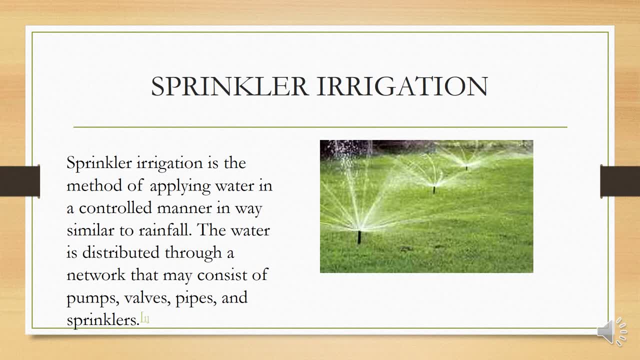 The water is distributed through a network that may consist of pump, valve, pipe and sprinklers. You must have seen sprinkler irrigation in the image. All of you must have seen it. So this is also one type. You must have seen it, mostly in the gardens. 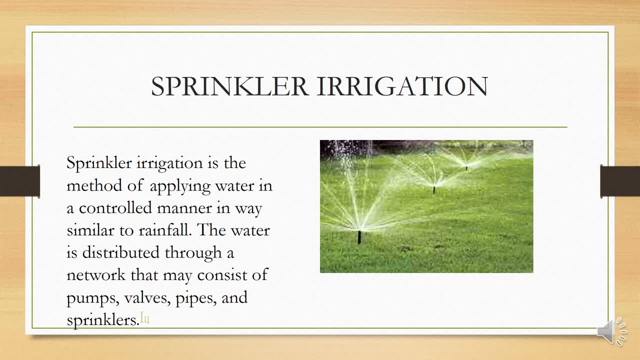 But this is also one type. We also use this sprinkler irrigation in the agriculture area, And why? Because it is in the form of rain, That is, the crop is provided with rain-like water. And which components are used in this? 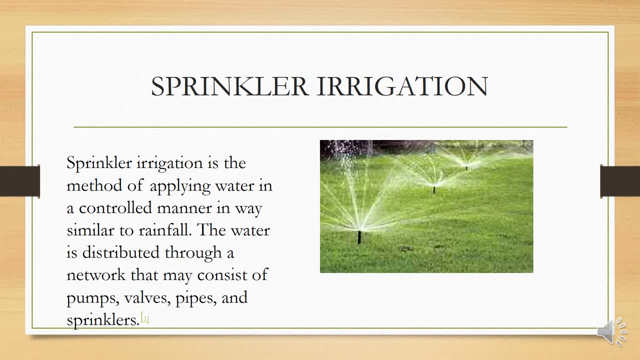 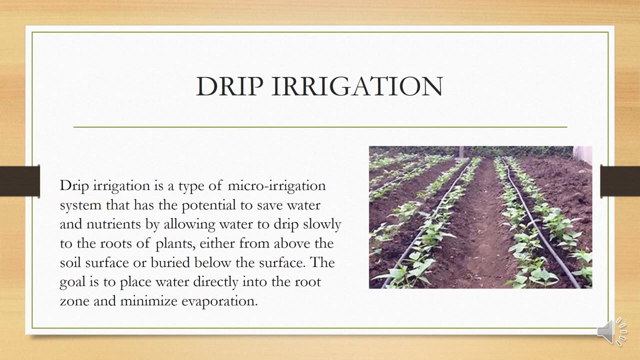 Pump, valve, pipe and sprinklers. Okay, This is also one of the most common types of irrigation. It is used in many places. The third type is drip irrigation. Drip irrigation is a type of micro irrigation system that has the potential to save water and nutrients by allowing water to drip slowly to the roots of the plant. 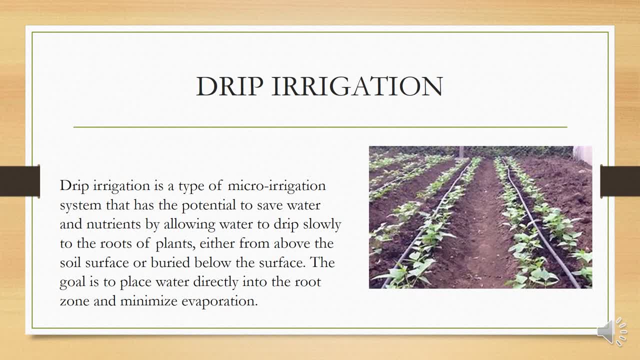 Either the form above the soil Or pure it below the surface. The goal is to place water directly into the root zone and minimize evaporation. Now, what is drip irrigation? You can see in the image that a pipeline is placed at the base of the plant, where its roots are. 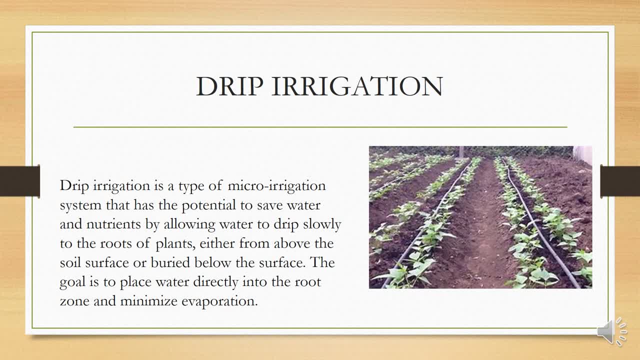 And this drip irrigation provides a very small amount of water. What happens with this? This is useful for which plant? For which? Because the water requirement is very low, It has a small amount of water requirement. And what happens with this? Whatever water is there, it is placed either on the surface of the soil or below the surface.